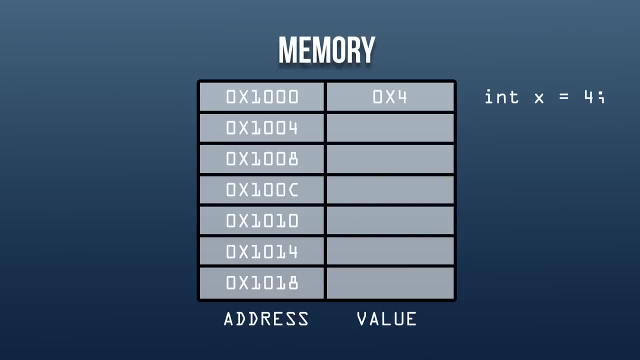 which gets allocated to that memory on the stack, and now that number lives there. So what happens now if at another location I put the number hex 1000 at address hex 1004?? I've just created a pointer. You may be thinking low-level learning. how is this possible? 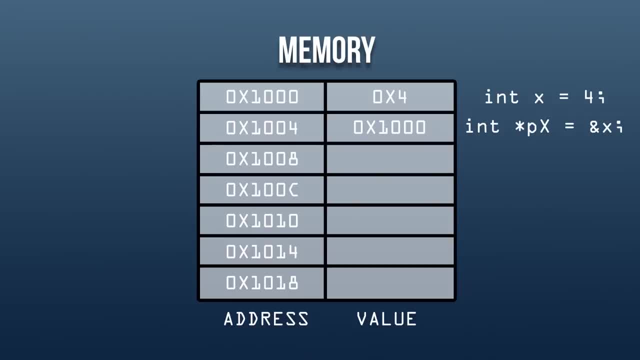 That's just a number at a location. Well guys, that's the secret. A pointer is just a value that happens to be an address. Mind blown, By setting the value of one variable equal to the address of another, that variable now points to the other. For new programmers, though, 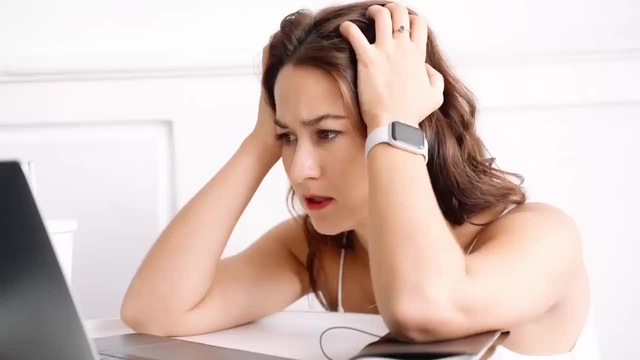 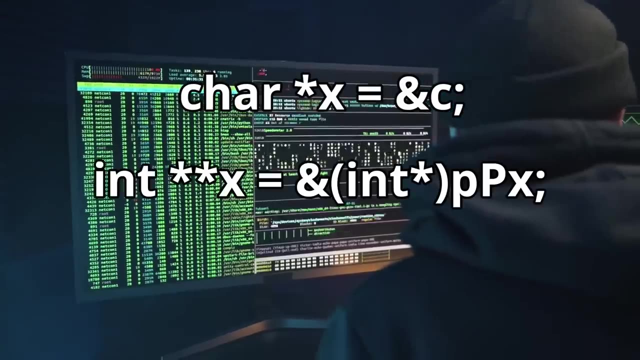 most of the time, that isn't as easy as it seems. One of the most common issues new programmers have with pointers is the syntax used to create them. The combination of stars and ampersands and arrows and more stars creates a lot of confusion, So let's break this down using our previous example. 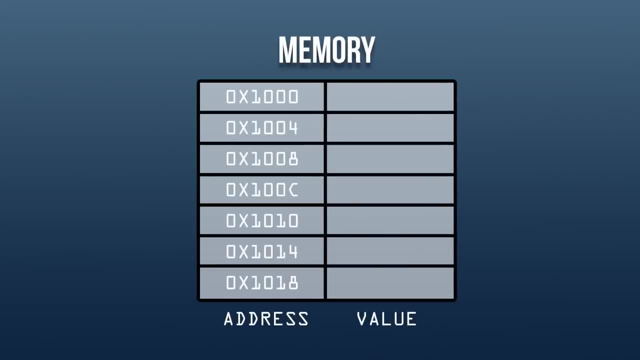 In our last example we made an integer x whose value was 4 at location hex 1000.. After that we made a pointer that lived at address hex 1004, whose value was hex 1000.. So how do we do that in C? We can do that using two lines of code. 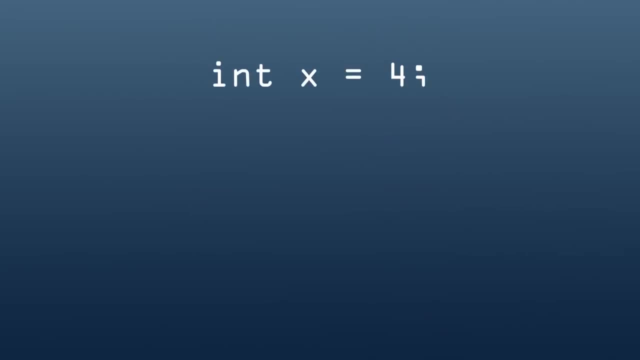 and I'll break them down part by part. The first line is: int x equals 4.. This line is pretty straightforward. The first part, integer, is the type of the variable: 4 bytes wide. This will matter later in the video. The second part is the name: Nothing. 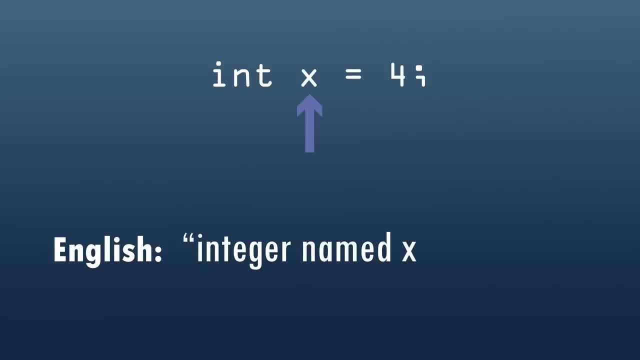 special here- just the variable name x, And then after that we put an equal sign which, when describing C, we can verbalize. the equal sign to is set to, And then finally the value 4.. So the final sentence we've come up with is: integer, whose name is x, is set to the value 4.. 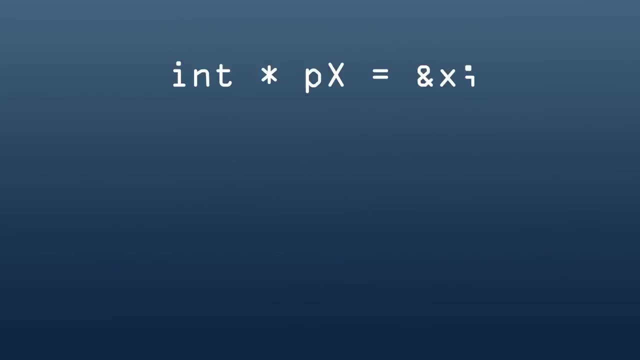 Okay, easy part over. Next is the hard part. To make a pointer to x like we did in our example, I've got to say the following line of C: Int. star px is equal to ampersand x. Now I know that sounds. 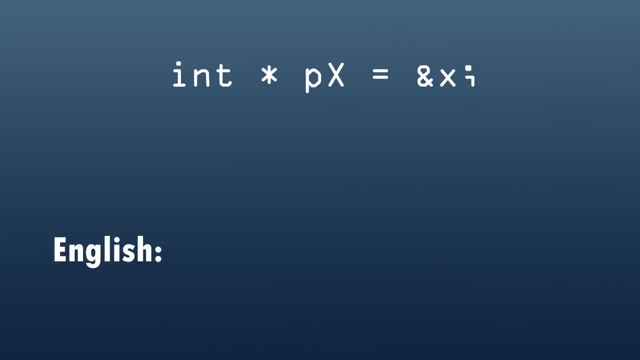 pretty crazy and a little scary. Let's break it down piece by piece. From left to right. we can see the type again, starting with int, Ah, but next we see the dreaded asterisk. What does that mean? When an asterisk is placed next to a type, it modifies the type. 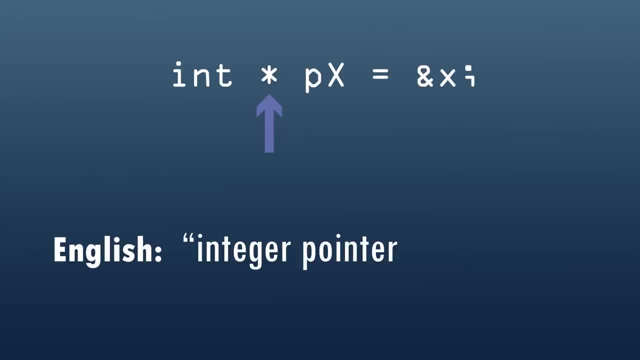 meaning that our variable is now a pointer to an integer. So our variable here points to a 4-byte value. Next, the variable's name, which is px or pointer to x. You can name it whatever you want, but this is a good habit: using p to denote that it's a pointer And then after that: 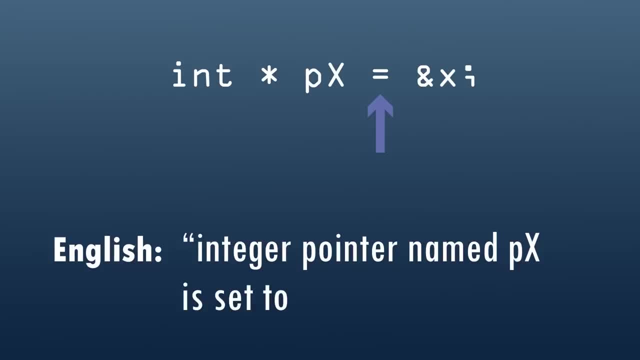 our equal sign, which again means, is set to Ah. and then the next dreaded character, the ampersand. Whenever you see an ampersand, just think in your head the address of. So this means the address of x. Our final sentence here is: int, pointer px. 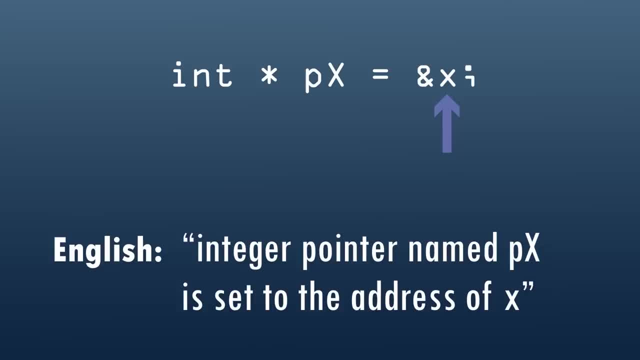 Is set to the address of x. So what does this do for us? Well, now, by using the pointer, we have a way of accessing x by reference instead of by value. So, for example, if we wanted to copy the value of x to a new variable using that pointer, we could do that pretty easily with. 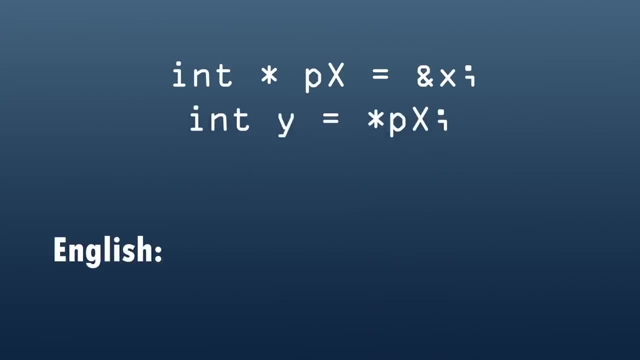 this new bit of code. We'll say that int y equals star px. Now what is this code doing? Let's break it down Again: y equals px. Now what is this code doing? Let's break it down Again: y equals. 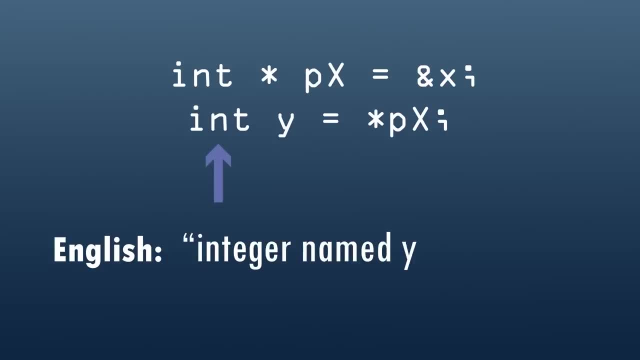 px. Now what is this code doing? Let's break it down Again: y equals px. Now what is this code doing? Just like x is a normal integer, so no pointers. yet We say that y is set to using that equal. 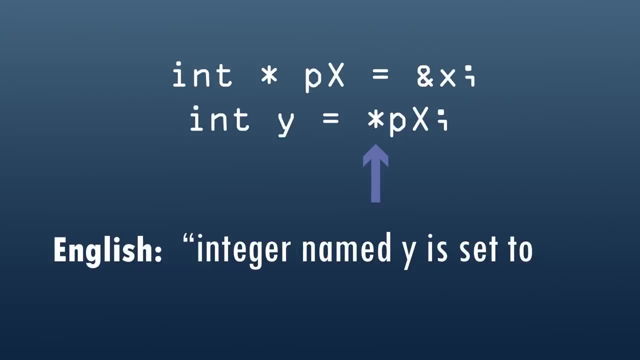 sign: Uh-oh, the asterisk again. Remember how last time I said, when we see an asterisk, it's used to modify a type if a type is near it. Well, here there is no type When it's used alone. 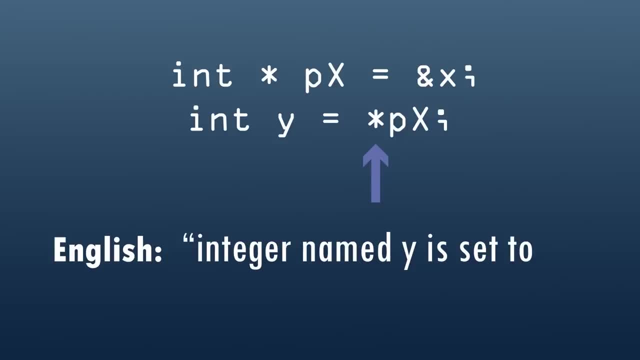 this way the asterisk is referred to as a dereference. The dereference means go to the address pointed to by the pointer and grab that value. So because the pointer is set to a new value, it's going to modify the type if a type is near it. So when we see a pointer we're going to 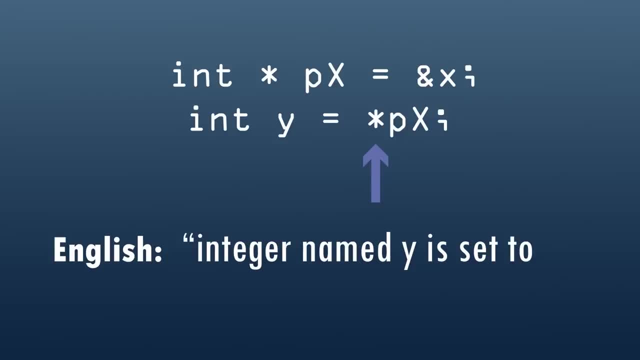 set y equal to x. So because px points to x, the dereference will go and grab that value and it will set y equal to x. So when we're verbalizing c, when you see an asterisk by itself, you can say the thing pointed to by. This would mean that the final verbalization of this line of 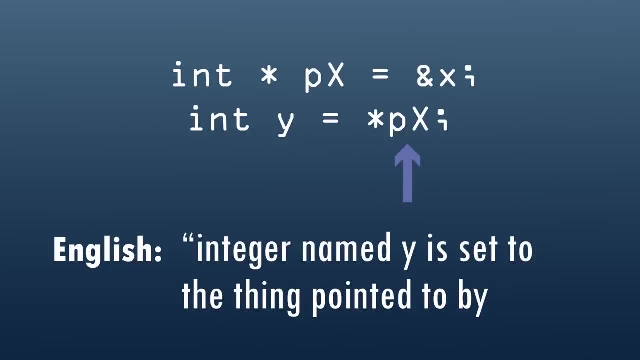 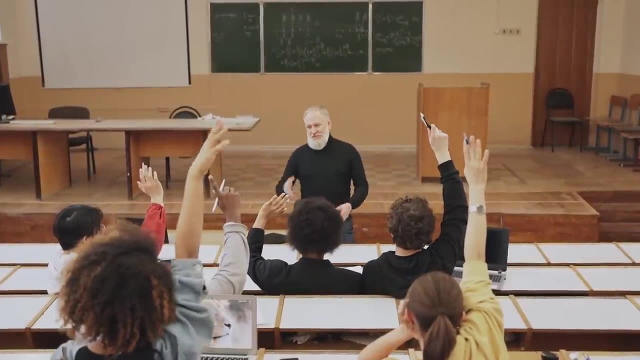 c is integer. y is set to the thing pointed to by px. By doing this we can pass around x by reference at a value, and why that matters I'll explain in the next part of the video. The final concept that confuses people the most when learning about pointers is: